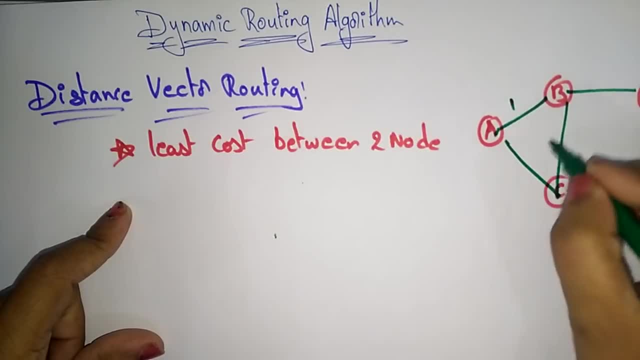 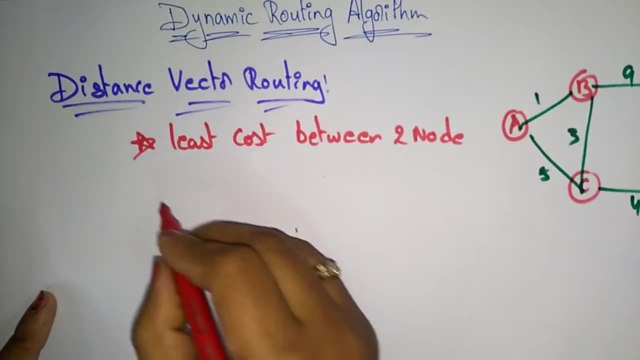 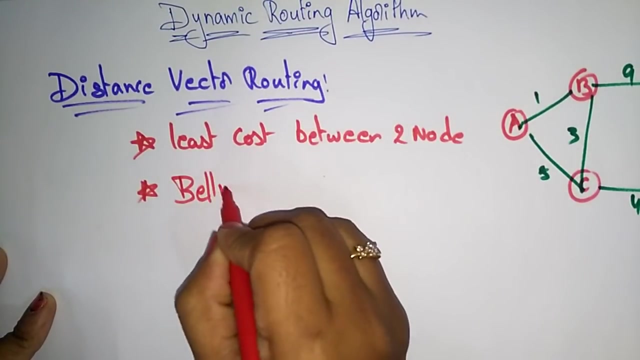 select the least cost between two nodes. so here the cost of the each node edge will be there. okay, let's see. and the second point is one of the example for the distance vector routing is a bellman ford algorithm. a bellman ford algorithm is a distance vector routing algorithm. 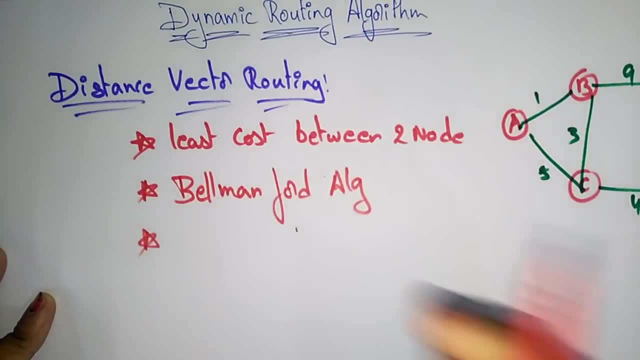 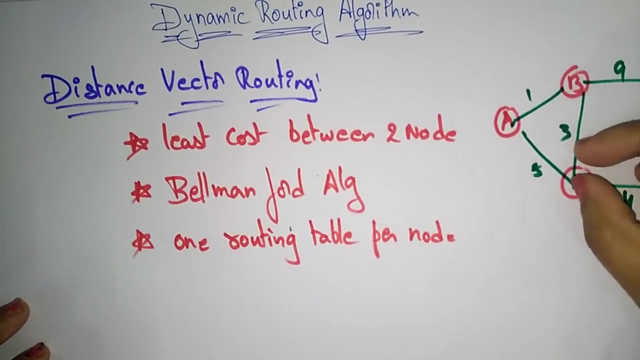 and here in dynamic routing algorithm or a bellman ford algorithm, we had to find out the routing table per each node. so one routing table per one node, one routing table per node. so, whatever the node you have taken, for each and every node we have to find out the 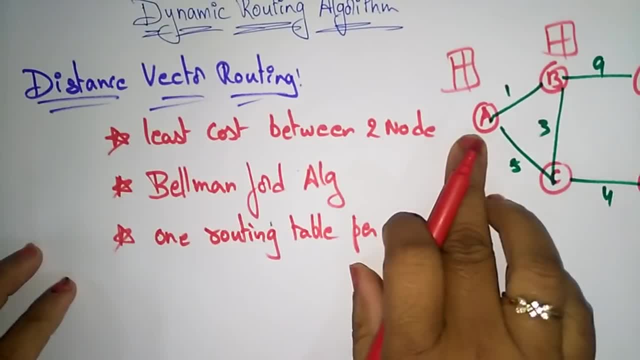 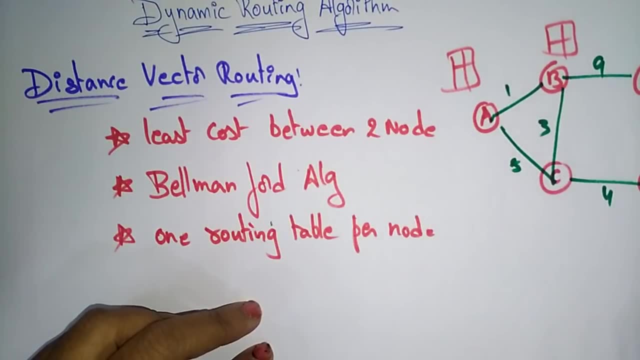 routing table. okay, means suppose if a is a source and this a wants to reach all the nodes. so if a wants to reach the nodes, whatever the node you have taken, for each and every node we have to, is a best path, means the least cost between those two nodes. and suppose a 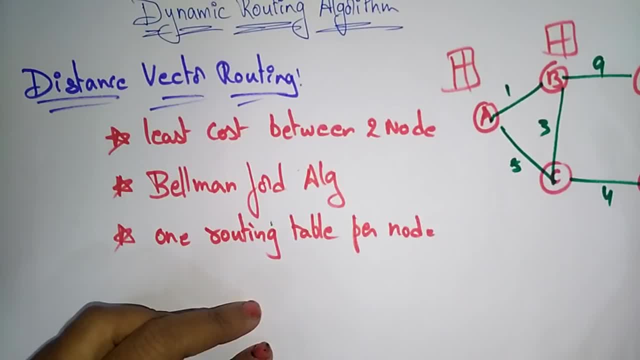 wants to reach, that be in this direction or in this direction, in two directions or they. so in these two directions. which direction is the best direction? okay, with less cost and up less traffic. so for each and every route node we have to find out the routing table. so with the help of that routing table the node can 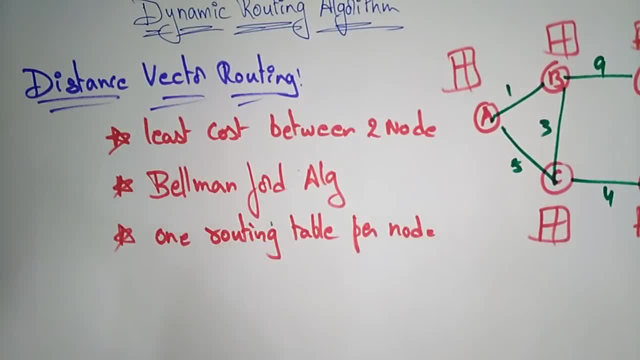 easily transfer the packet from whatever the destination it wants to send. suppose B wants to send the packet, so it has. it has some information like: suppose I want to send the packet to a, what, what is exact route, the correct room, and if I want to send the packet to 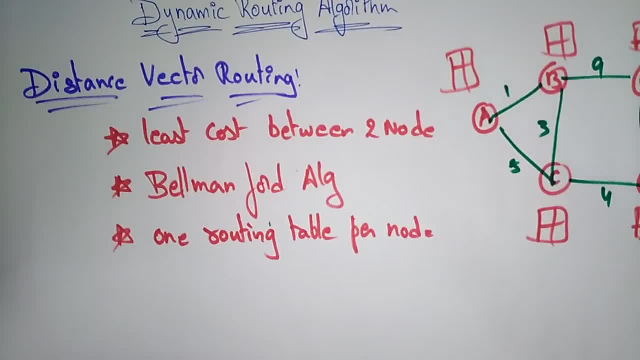 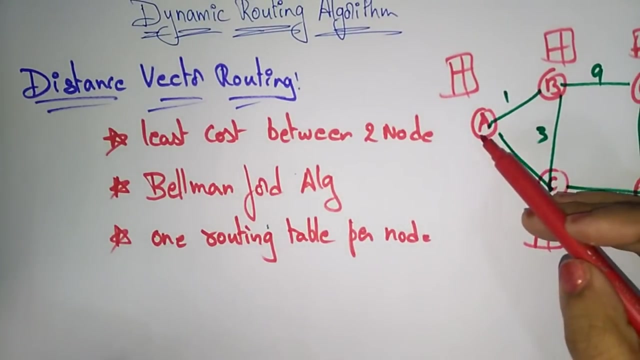 the D and what is the exact route I have to be followed. so that is a routing table. that B table consists of everything, information regarding all the nodes, okay, the path to all the nodes. so a address, c address, d address, e address, like that, suppose, if a routing 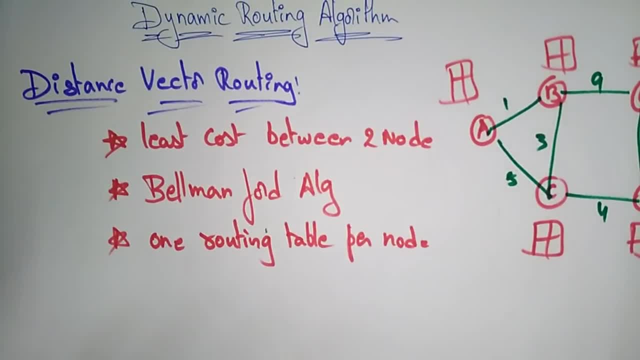 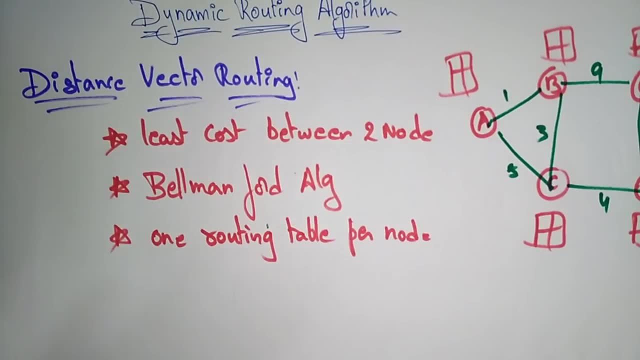 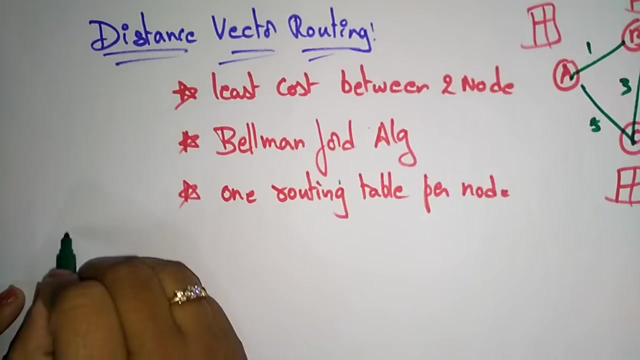 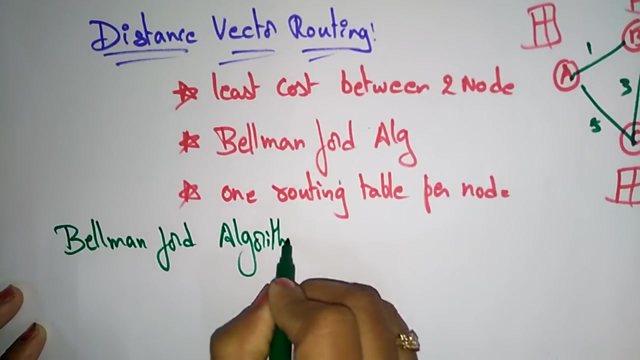 table. it is having the information regarding all the nodes so that we have to be find out. so that is a distance vector routing. so here in the distance vector routing, let's take the bellman ford algorithm. so the bellman ford algorithm defines: okay formula. is there, based on the formula, we are finding out the routing table for each and. 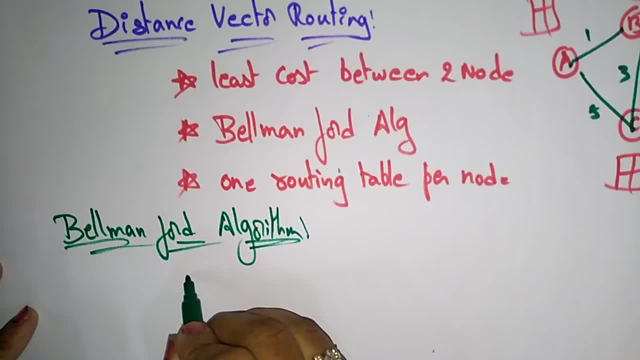 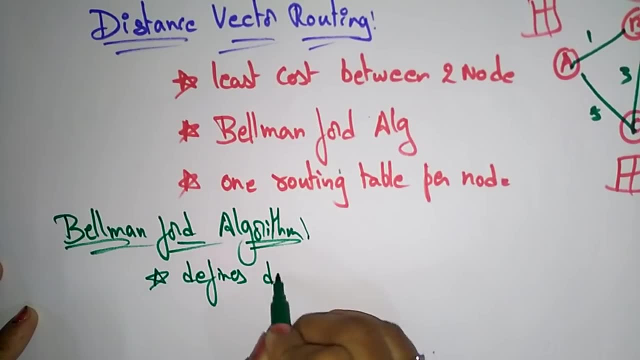 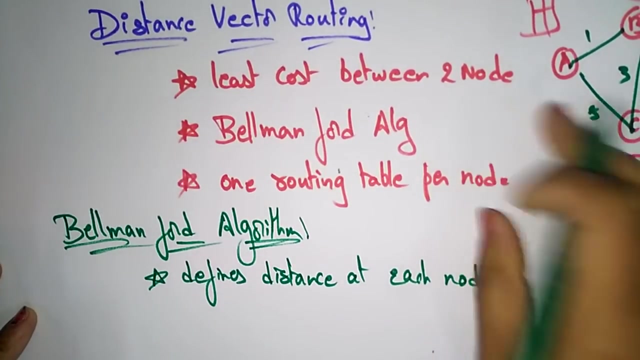 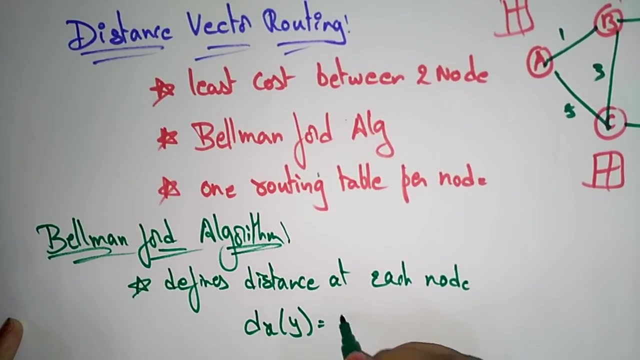 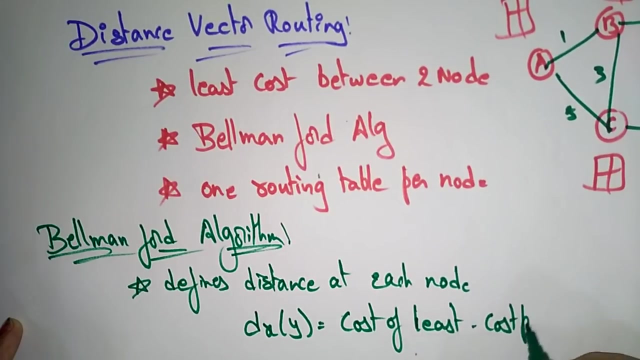 every node. so the bellman ford algorithm here it defines the distance at each node, defines distance at each node. so whatever the node you are selected- a or c or b- it defines the distance at each node. that is d. x of y is equal to cost of least cost path from x to y. so that is a, it defines the distance at each node. 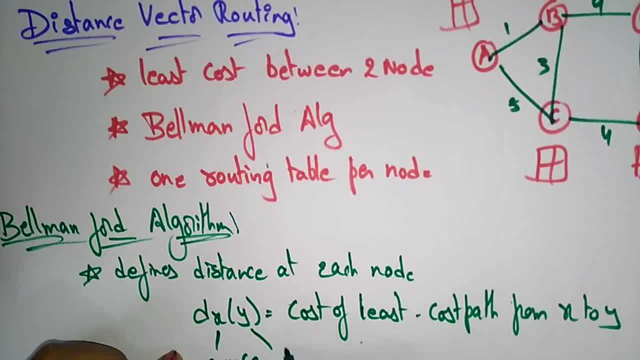 so here x is a source and y is the destination, so it defines the distance at each node. suppose i, x is a source and y is the destination i want to reach from x to y. uh, the normal distance is the cost of least cost path from x to y, so x to y. suppose i want to reach a to b, so a is. 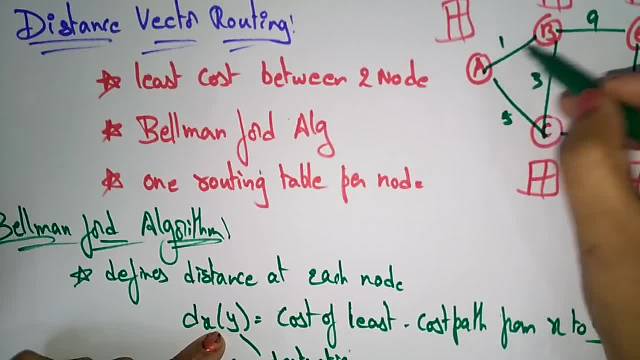 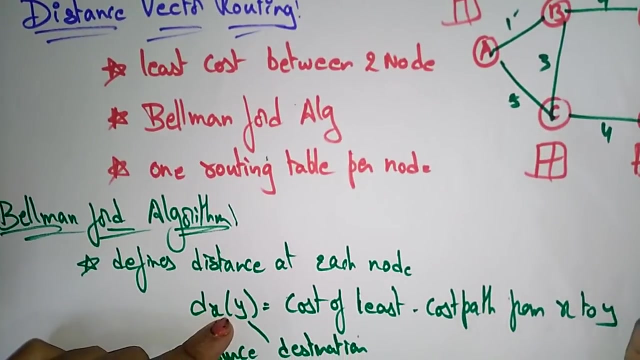 source and b is the destination. the least cost path for x to y is one. okay, that defines the dx of y, suppose it here. another root is z, 5, going to c by taking the intermediate node help, and going to b. so 5 plus 3, here 8. so the distance of this path is more so i i just select this path so like: 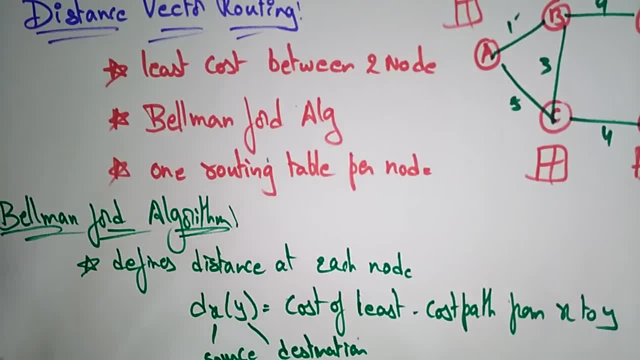 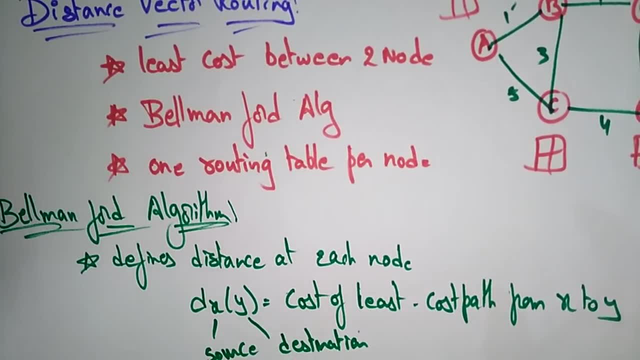 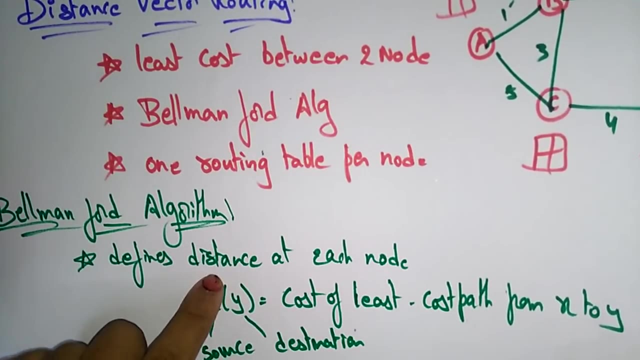 that. so this is, this can be done in manually, okay, so with the help of the formula, you can easily calculate the distance. which node is the best node? okay, uh, to try which node, we have to take it as a intermediate node to reach the destination. so define the bellman for algorithm. defines the. 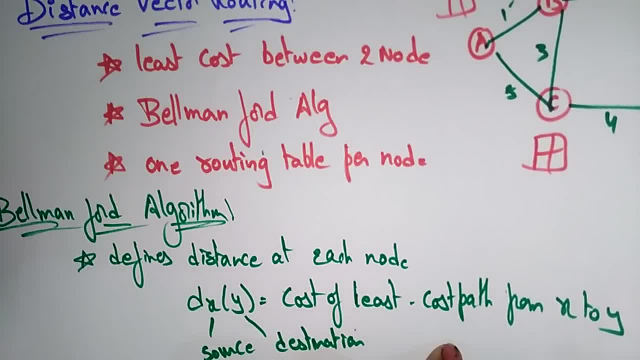 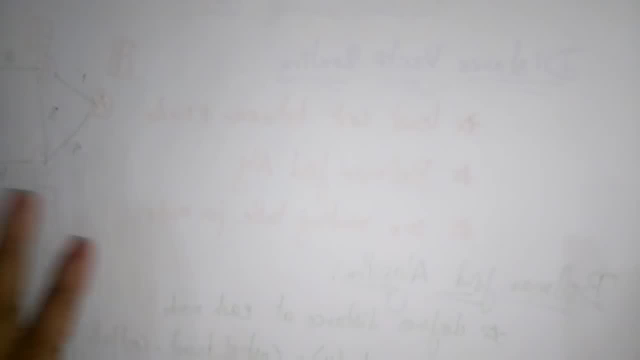 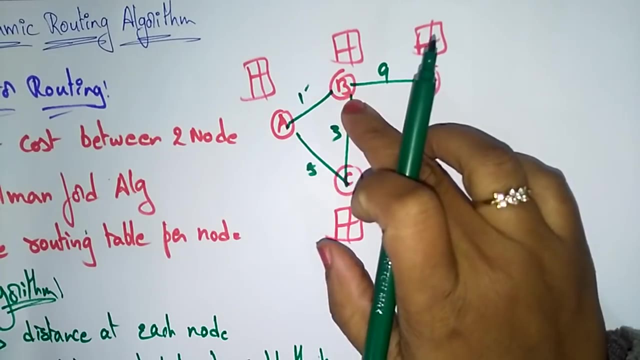 distance at each node. d, x, y is the cost of least cost part from x to y and update distance based on neighbors also. so suppose, if you consider the neighbors here i just taken b as a my, so here the source and the destination. there is no intermediate nodes and i didn't check. 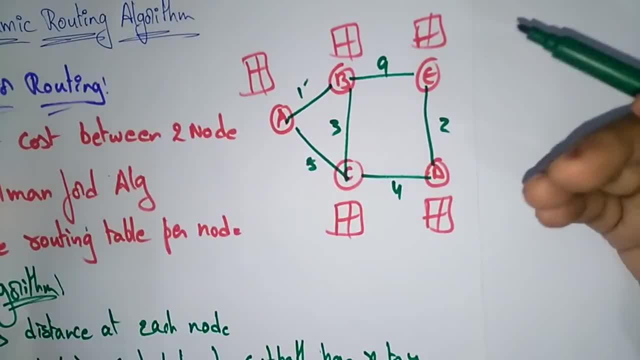 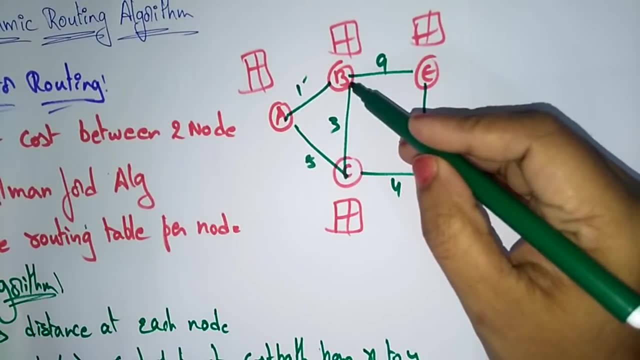 any neighbors, suppose if, if you want to check the neighbor nodes also, i want to check the c also. okay, so let's take here it is a five and here one and two, this distance will be less so update distance based on all neighbors you have to be. 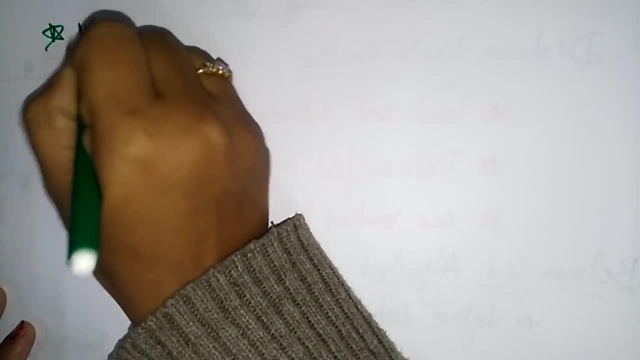 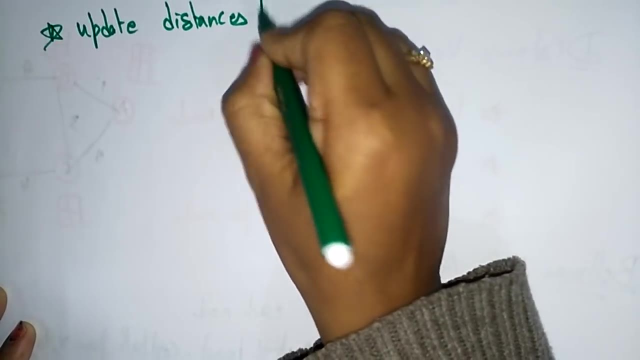 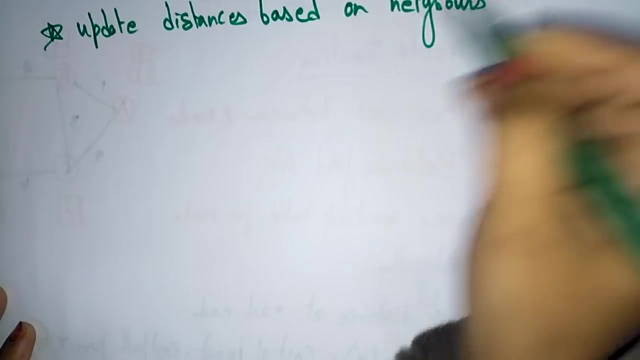 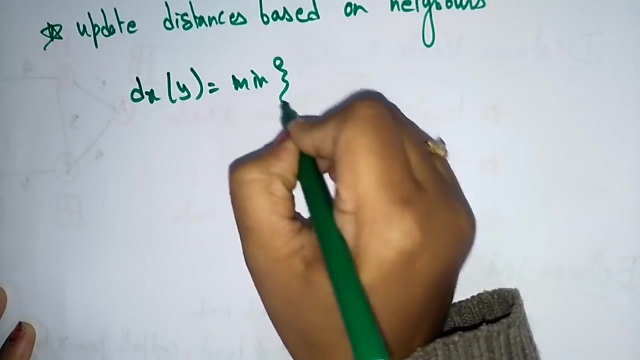 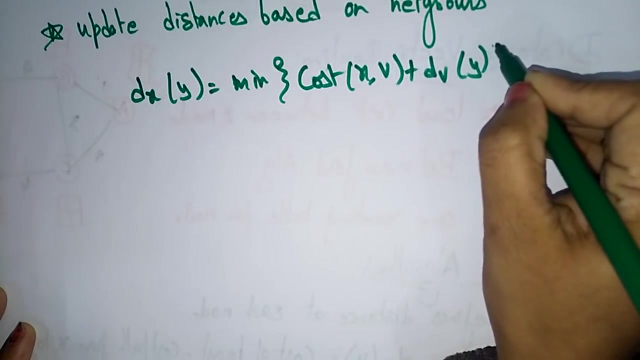 calculated. so the formula for that is update distance, update distance based on neighbors. so, based on the neighbors, what is the update distance? the formula was this: dx of y is equal to minimum of cost, x, comma, v plus dv of y. so this is the updated distance based on the neighbor. so whatever the node you are selected, 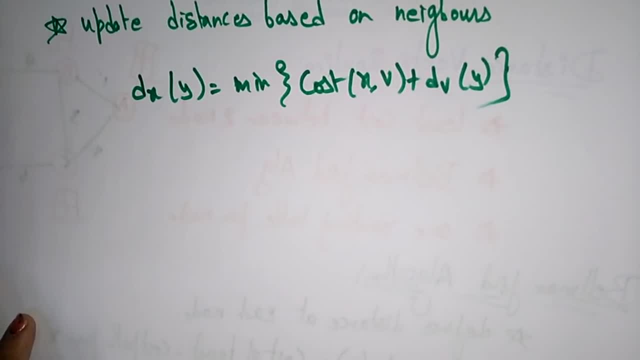 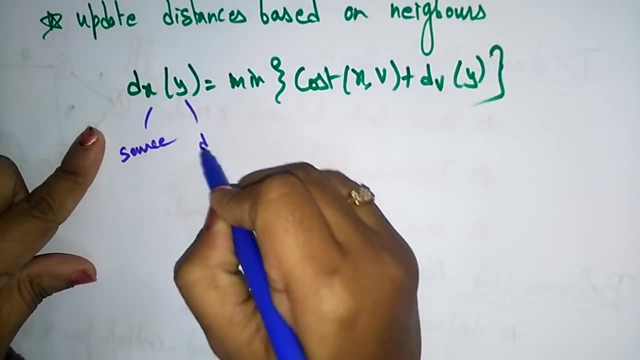 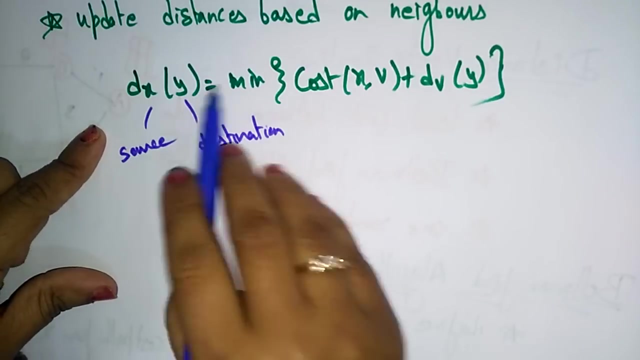 okay, for that node you have to consider all the neighbors also. so neighboring nodes also: dx, y. x is the source, i said, y is the destination. if you want to go from x to y, if you want to find the path from x to y, the formula for is by considering all the neighboring nodes. 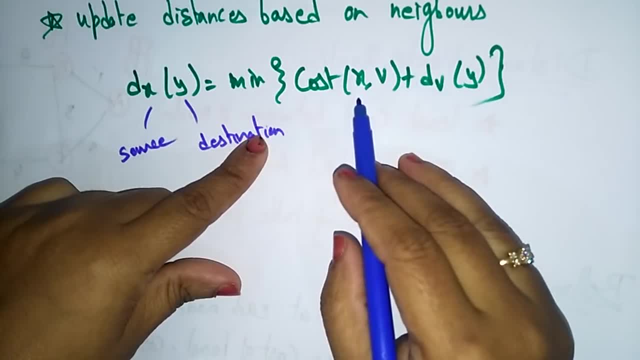 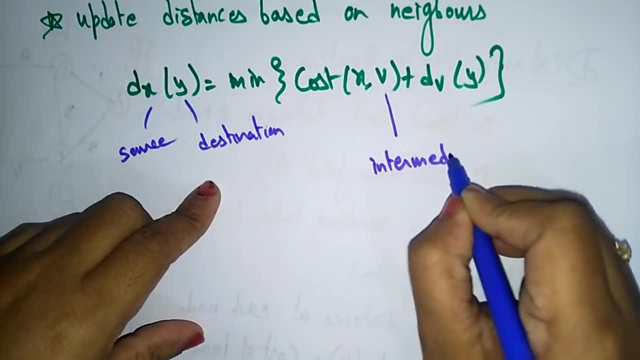 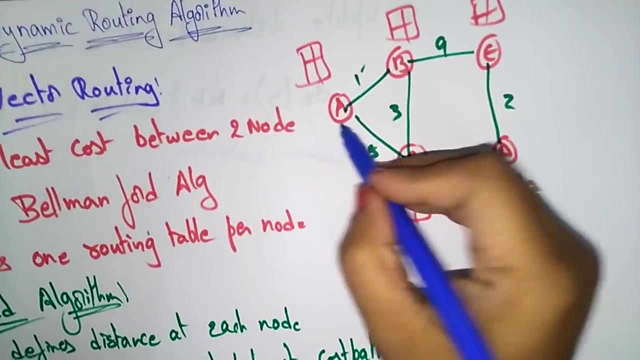 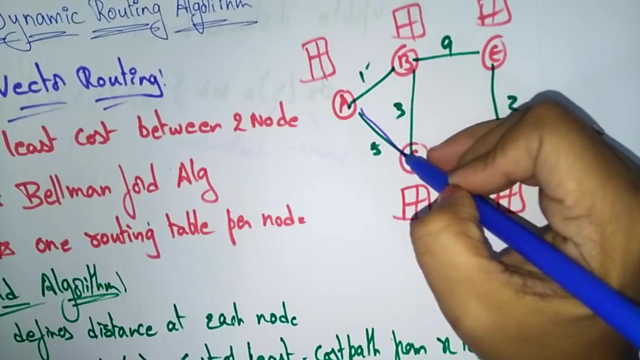 minimum of cost of x comma. v. x is the source, i said, and whatever the v, v is nothing but the intermediate node, intermediate node. so here, in this example, a is the source and suppose b is the destination. what is the intermediate node here? c is the intermediate node. suppose if you want to travel in this way, c acts as an intermediate node. means: 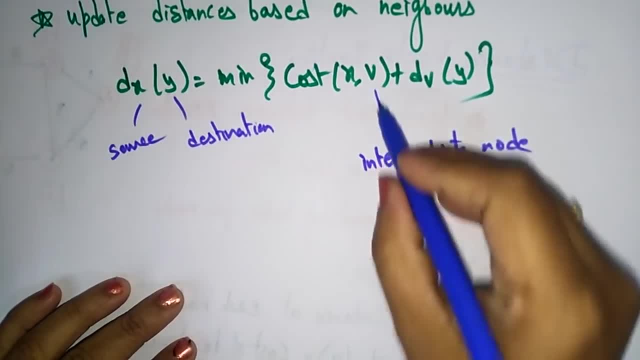 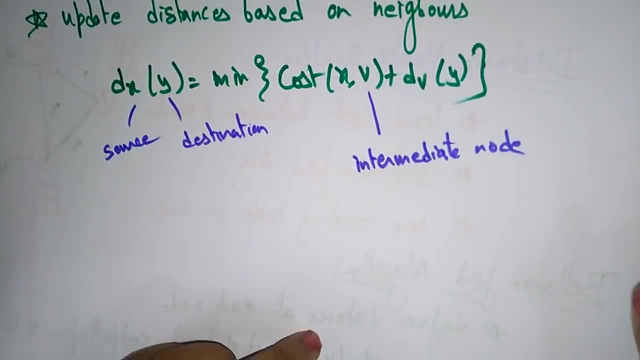 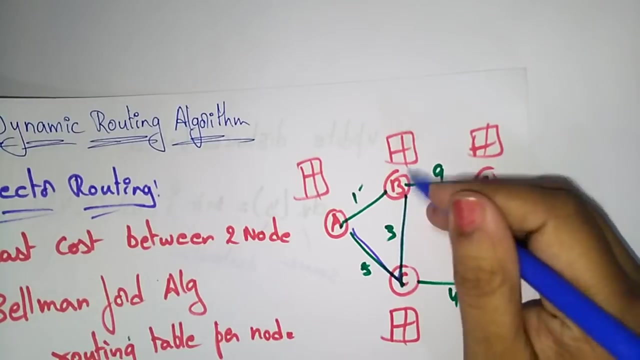 this is v, that is nothing but v. so v is the intermediate node and dy of v is the destination path, the value of y. so what is the value of y here? dv of y means this: three distance of y. so this is the intermediate node. this intermediate node is reaching the destination and that 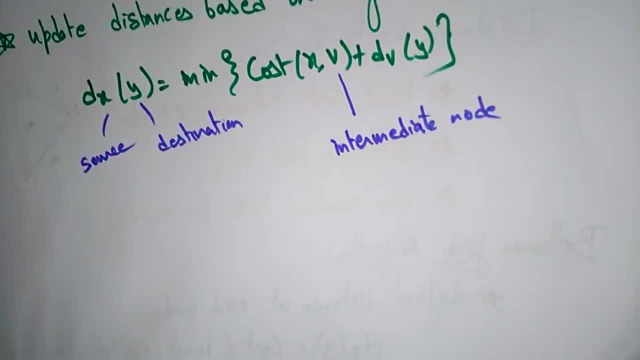 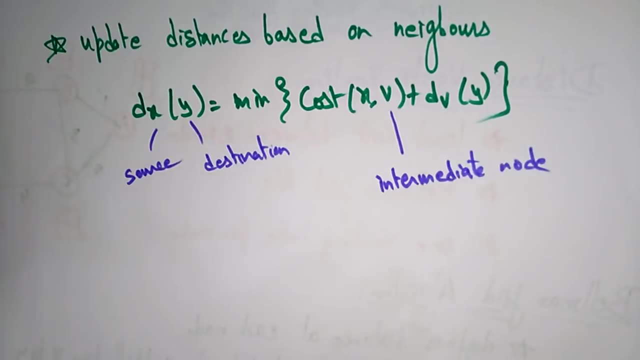 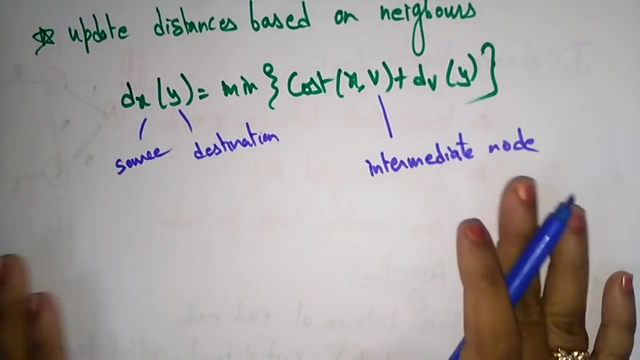 value is this: that is a dv of y. okay, so this is a formula for bellman's for algorithm. now apply this bellman for algorithm and we have to find the distance vector routing for each and every node. so let us take here in this example. i just want to explain you by taking 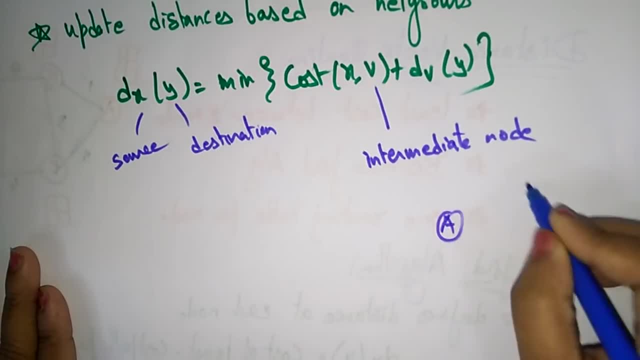 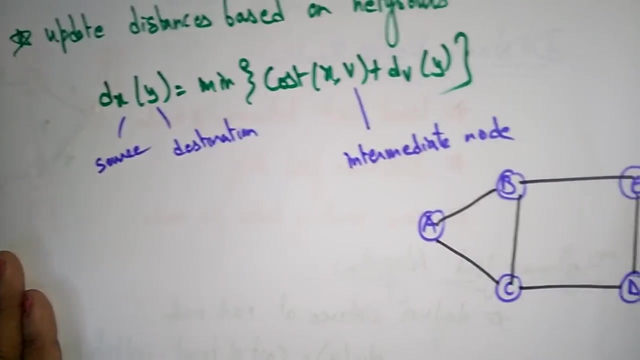 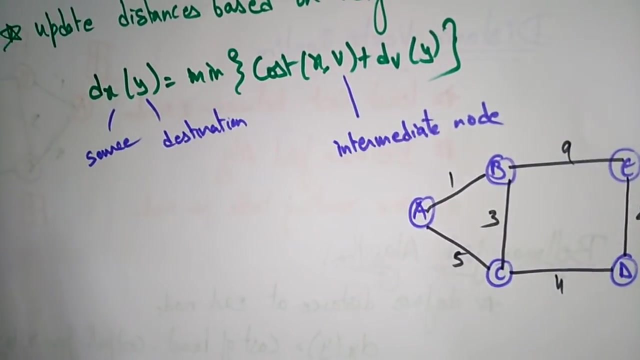 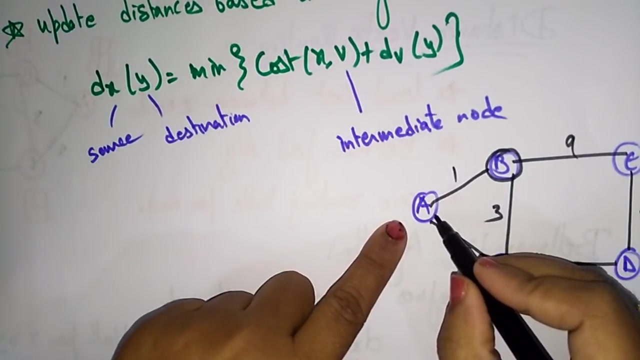 one node as an example: a, b, c, d, e. okay, so here, this is the path and these are the values. okay, so let us take b as a source. let's take this b as a source and b to a. we had to find out the path, okay. 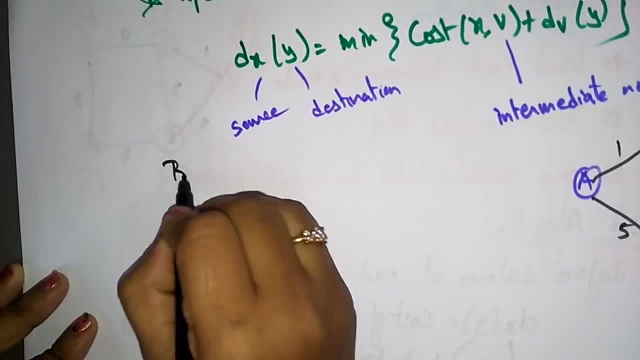 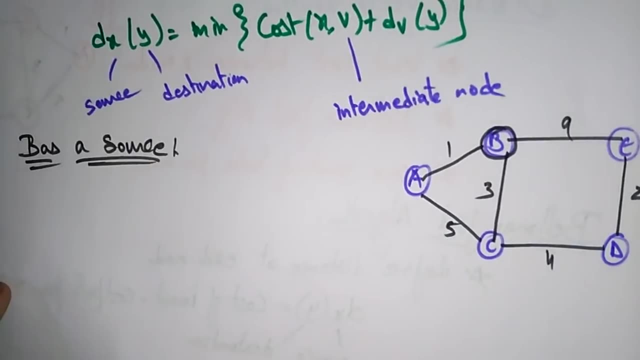 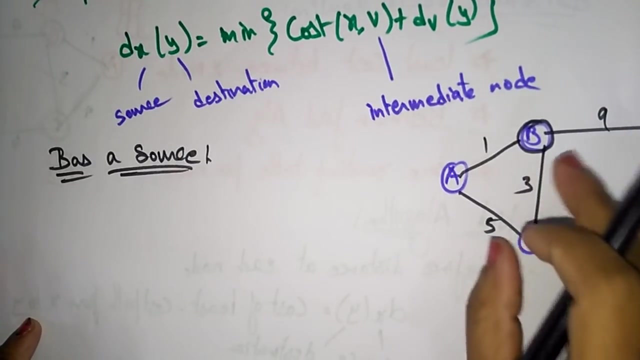 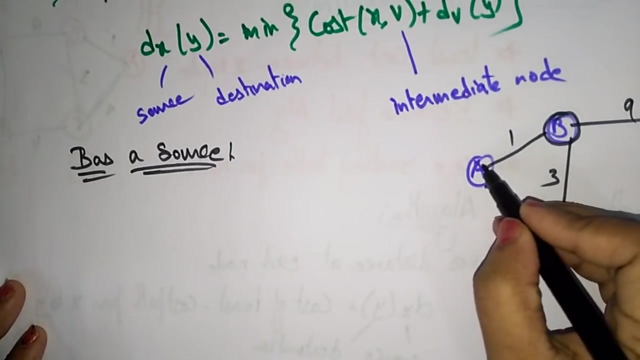 B as a source and A is a destination. Let us take B as a source. So if B as a source, what are the possible paths? that B consisting of Means? we have to find out the routing table for B. Let me find out the routing table for the B. Let us take first path B to A. 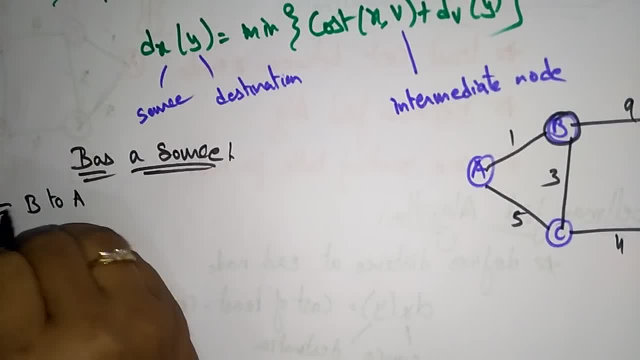 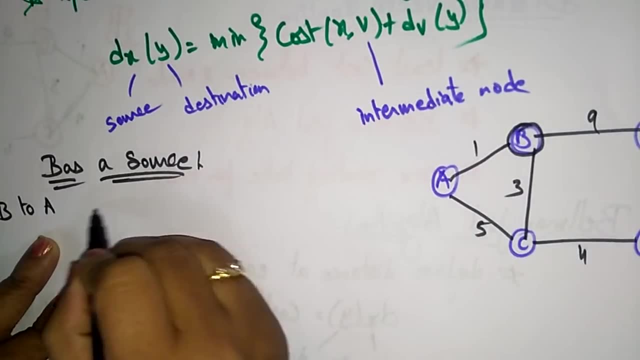 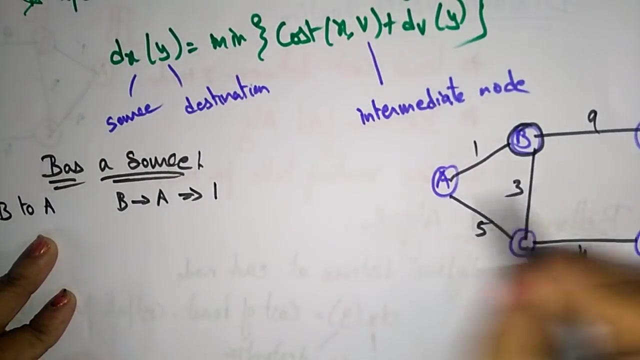 B to A. So what are the possible paths for B to A? One is B to A, B to A. what is the value? 1. And you can reach the B by taking the intermediate node. also B, C, A, This. 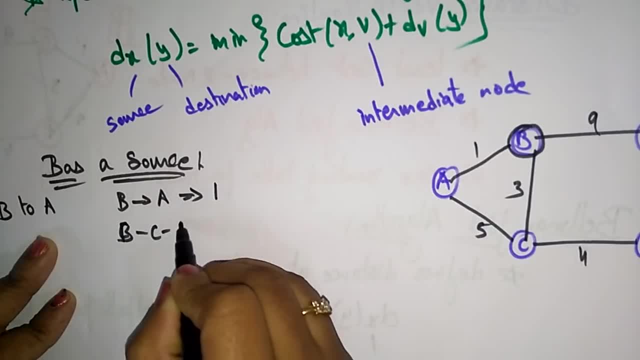 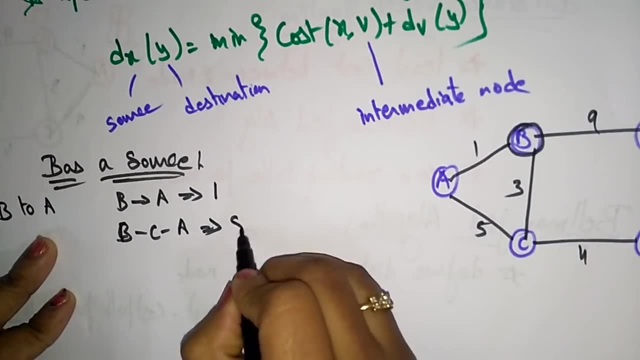 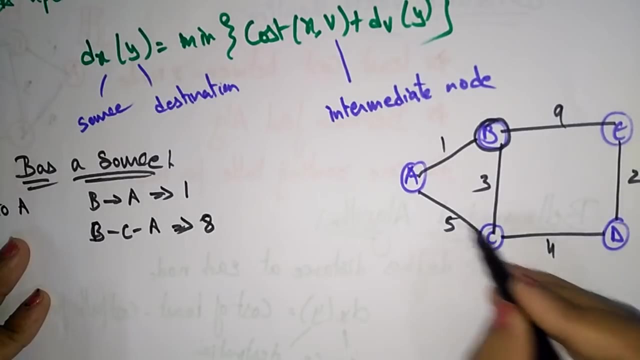 is another way: B C, A. What is the value of B C, A, 3. 3 plus 5.. Okay, So, 3 plus 5, 8. And you can reach A by taking this help: B, E, D, C. 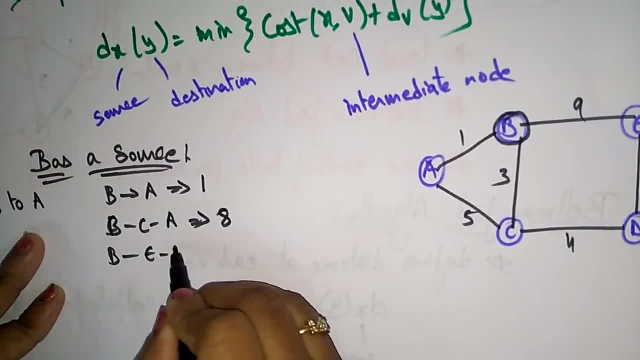 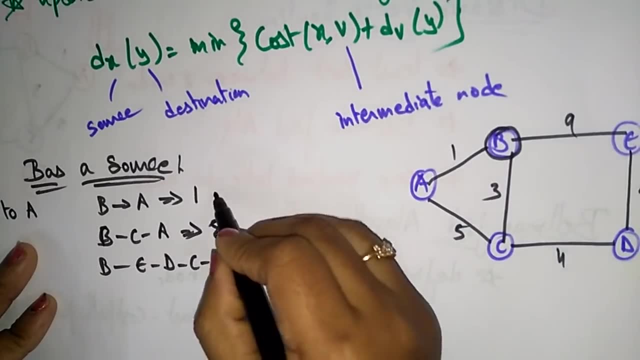 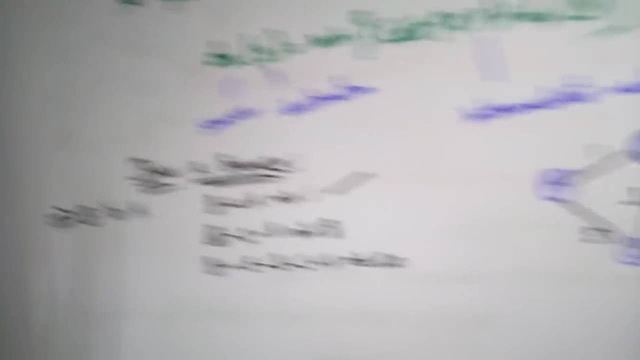 A. This is another way. B, E, D, C, A. The value of this is 20.. So, which is a minimum? This one is a minimum, So the table consisting of B to A. Let me take the table. 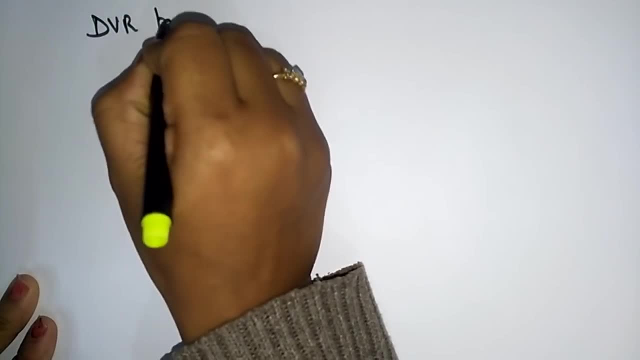 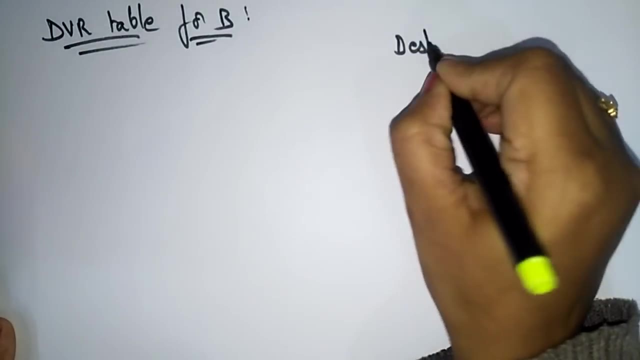 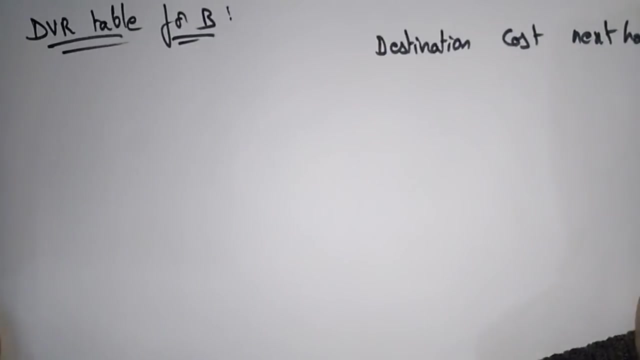 So distance vector routing table for B: Okay, Destination cost and next hop. Next hop is nothing but the next intermediate node. So what is the next intermediate node where data is transmitted? By taking with the help of that node, the data is transmitting. So let's. 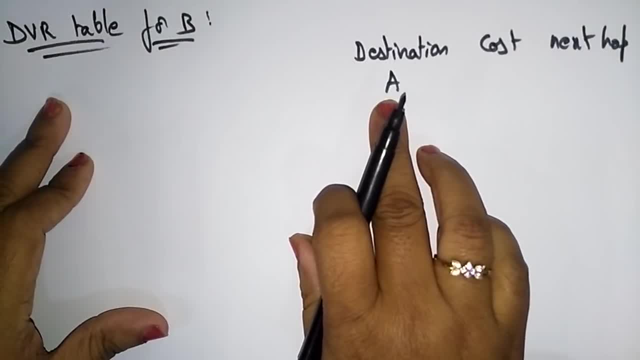 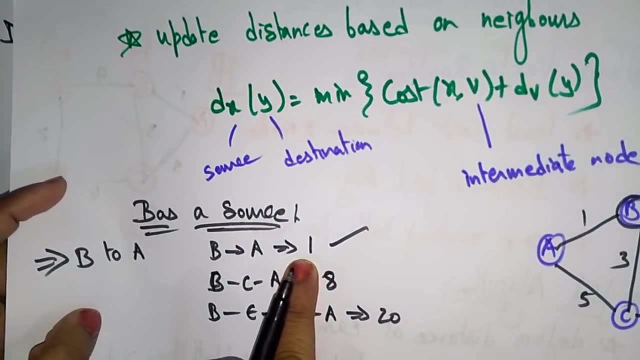 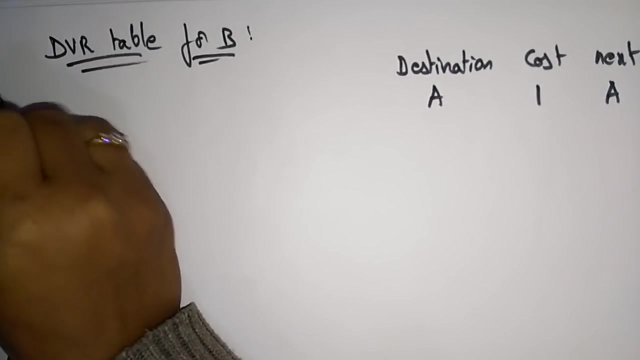 take B to A, find out. So A is the destination. Okay, So here, B to A. A is the destination. What is the minimum cost to reach that destination? 1. Okay, Next hop A itself. Now let's consider B to C, B to C. Let me draw the diagram again. 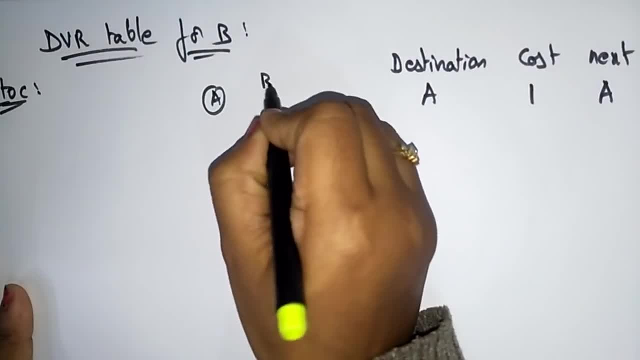 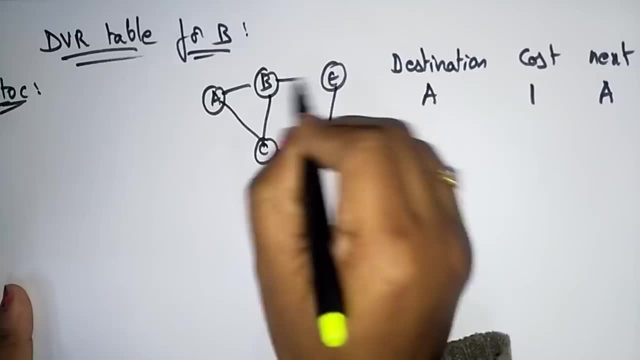 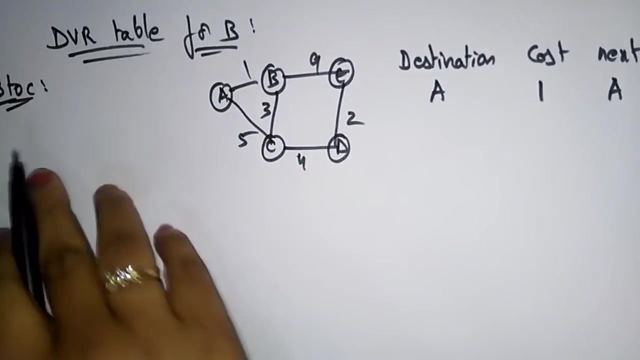 here, so that you won't be confused: A, B, C, D, E. Okay, And the values here is 1,, 3,, 5,, 4,, 9, 2.. Okay Now, C is the destination, B is the source. 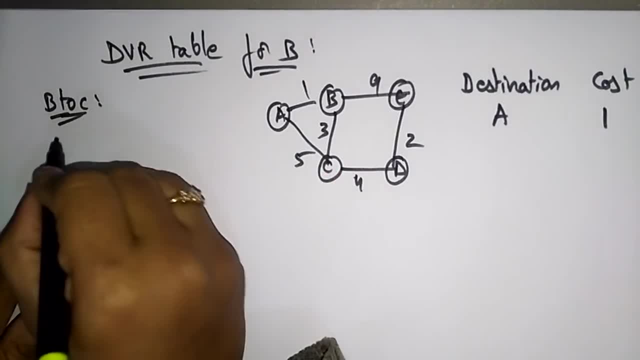 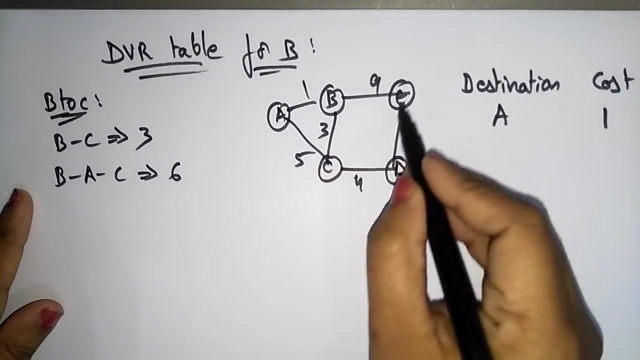 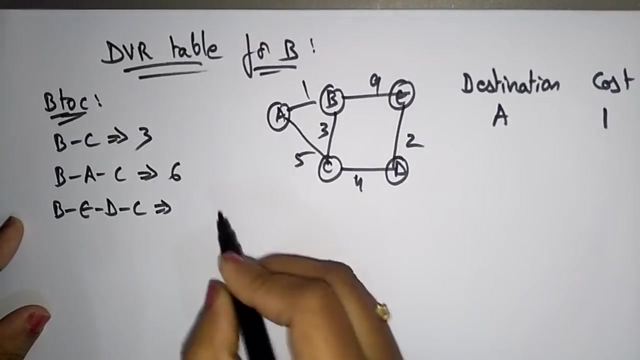 Okay, Now C is the destination. What are the paths that are available here? B to C is 3 directly. I can go like this also: B to A to C: 1 plus 5.. So 6.. go in this way also: B, E, D, C, 9 plus 2 plus 4, I will get the 15. So which is the minimum cost? 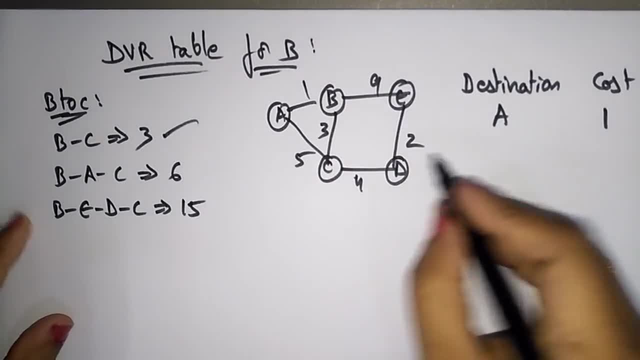 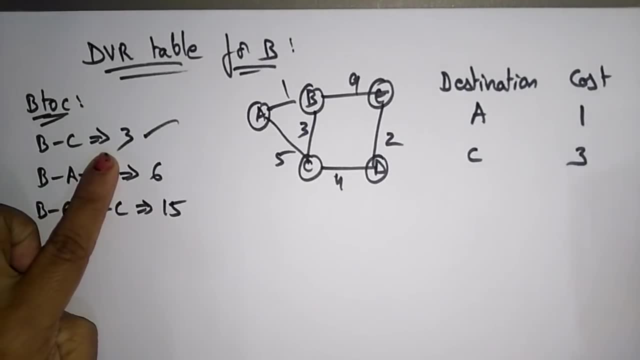 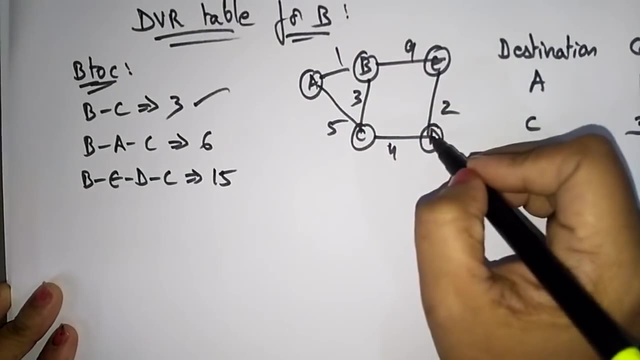 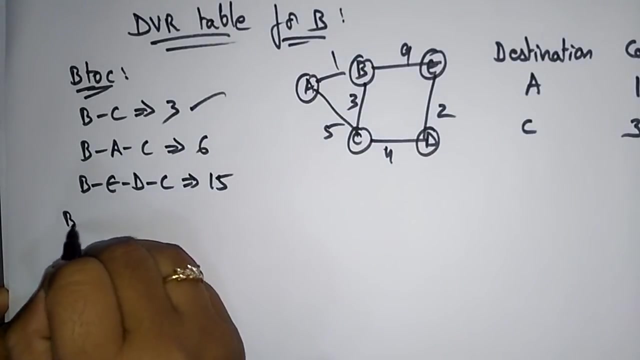 to reach the C 3.. Okay, So the destination: to reach the destination C, the cost is 3 and the next hope means the intermediate node, C itself. Okay So next let us take D is the destination, B is a source. This is a DVR table for the B only. So let us take B to D, or else you directly. 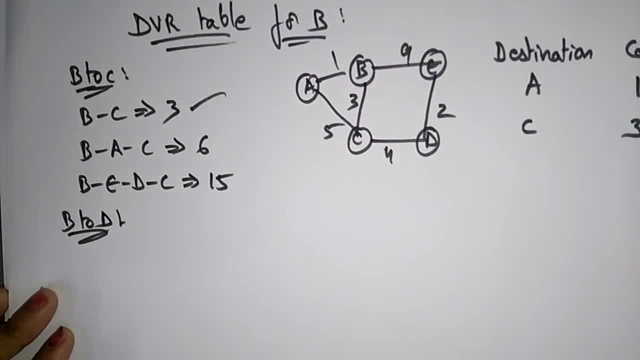 apply the formula. Okay, So that is the. what is the formula I had explained? Dx of Y means X is a source, B and Y is the destination and the minimum cost of X, comma, Y, the intermediate node, that is having, Okay, 9 plus 2, like that. you need to be calculated From that. you need to find the 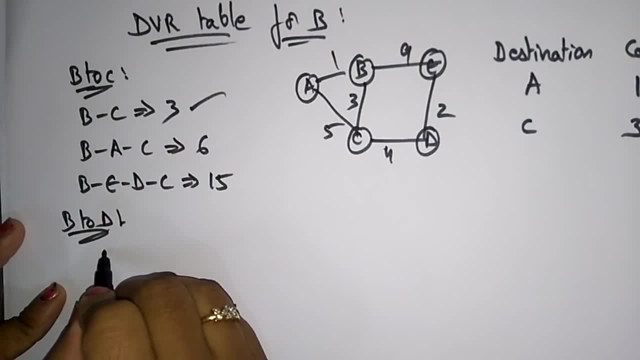 minimum cost of X comma Y. So this is the minimum cost of X comma Y. So this is the minimum cost of value. or else you just simply find out. So B to D, you can go B, A, C, D, So this is one root. 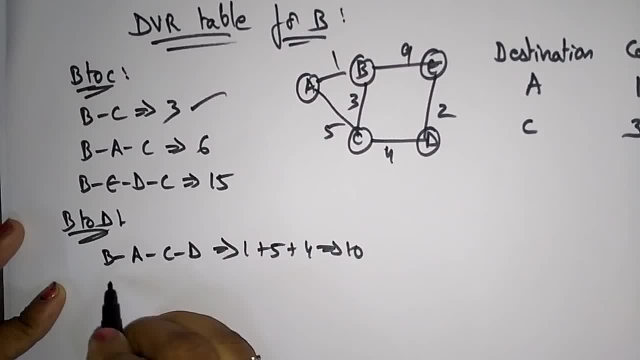 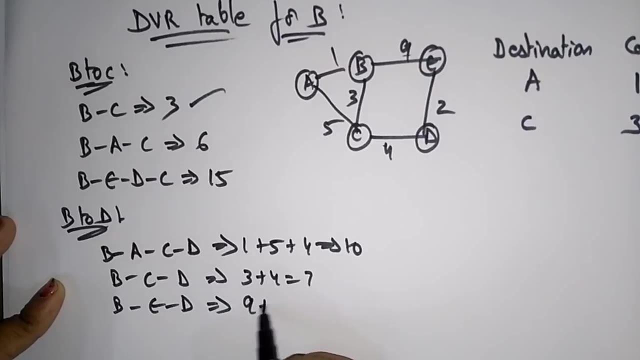 1 plus 5 plus 4, you will get the 10, and another root is B C, B C D- This is another root. 3 plus 4 is a 7, and another root, this one B E D, B E D, 9 plus 2, 11.. In this, 7 is the minimum. 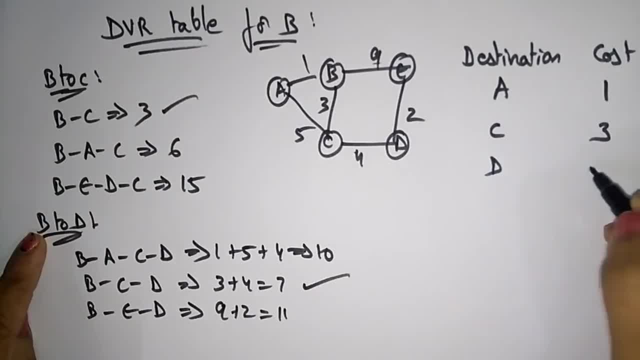 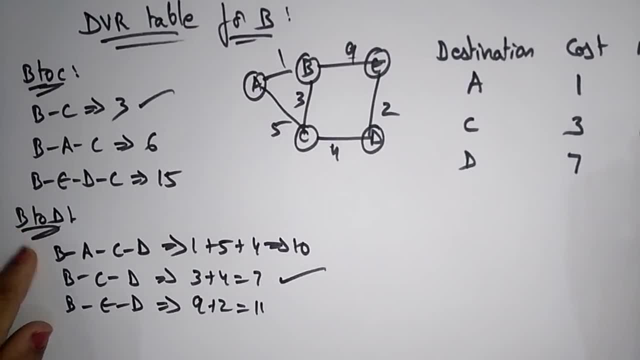 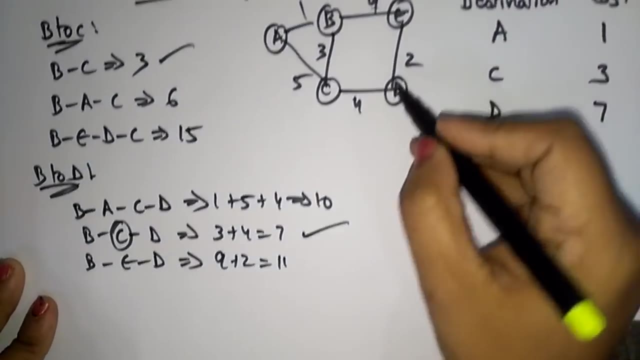 cost. So suppose the destination is D, the cost of travelling to destination to reach the destination D is 7. and the next hope, that is the intermediate node, is: what is the intermediate node here? C is the intermediate node. Okay, In the same way, if you want to reach the destination, 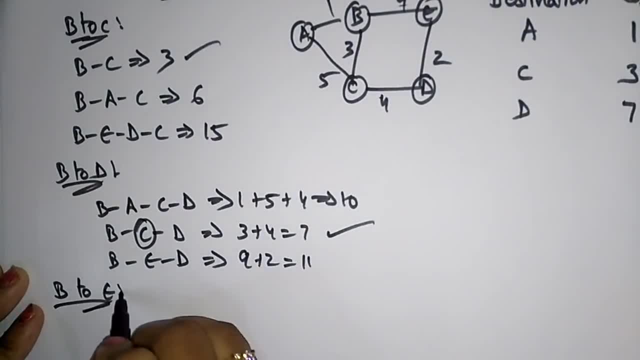 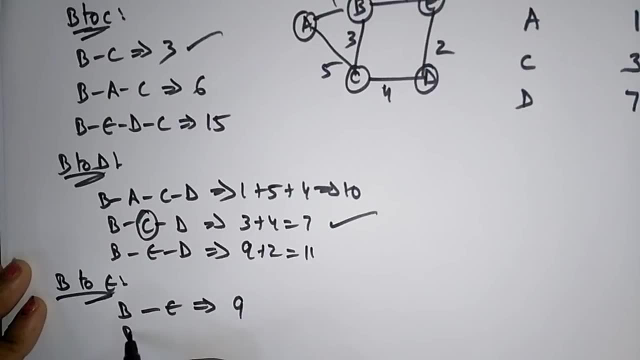 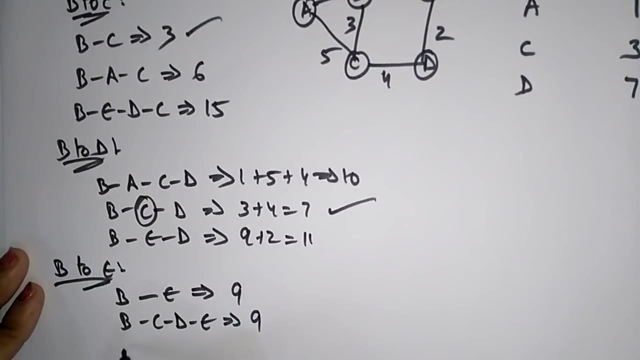 E, B to E. So what are the different paths? B to E is 9,. one direction, B to C, to D to E, you will get 9.. Okay, So this is another direction, and B to A, to C, to D to E, you. 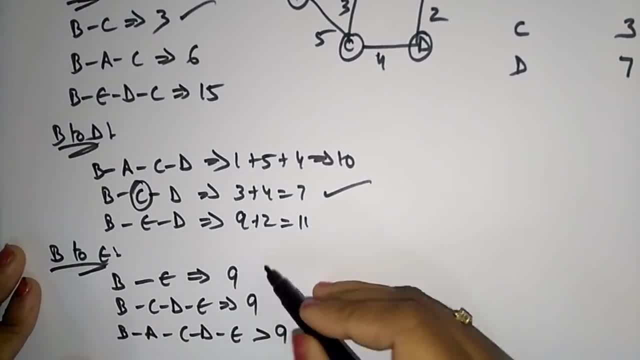 will get, it's more than 9.. Okay, So here you will get these two values as a same cost. So which one you need to be selected? So, while selecting the path, the thing is we have to take the shortest path as well as the short. 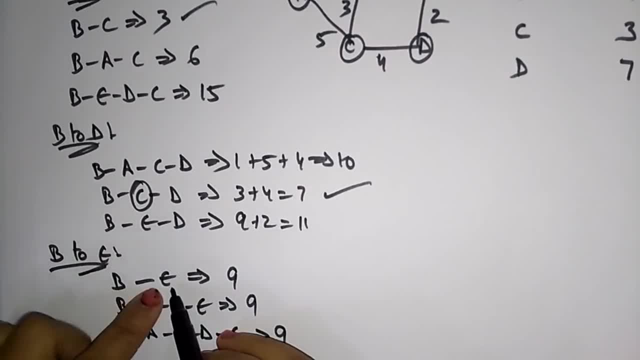 Less intermediate nodes, less nodes. So here, with the help of no, there is no intermediate node, here, two intermediate nodes. So it's better to take only this. B to E means the direct destination, source to destination. There are no intermediate nodes are present. Okay, So B to E. 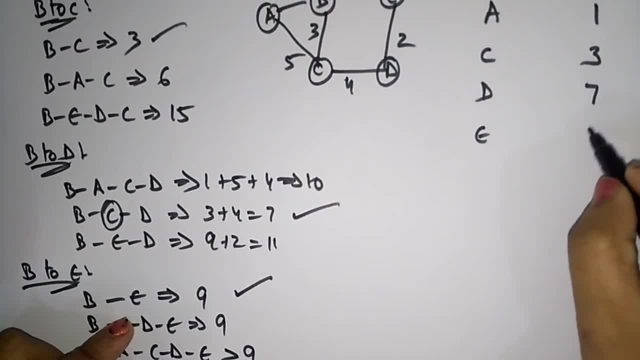 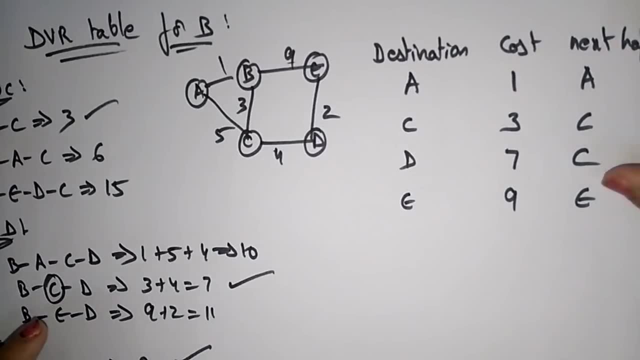 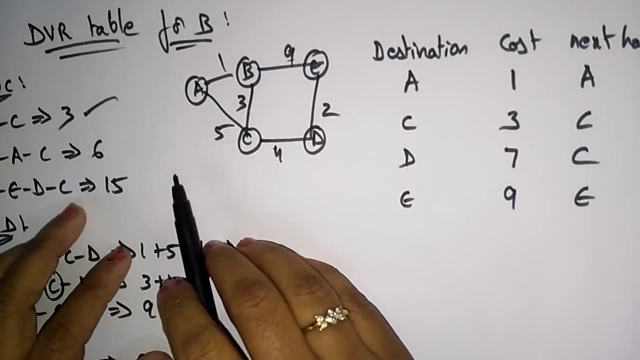 suppose E is the destination and the cost to travel to the E is 9 and the intermediate node is E itself. So this is a distance vector Table for B, only Like that you need to be calculated. that E table for distance vector table means one routing table for each and every node, for B, for A, for C, for E and for D, For all the.